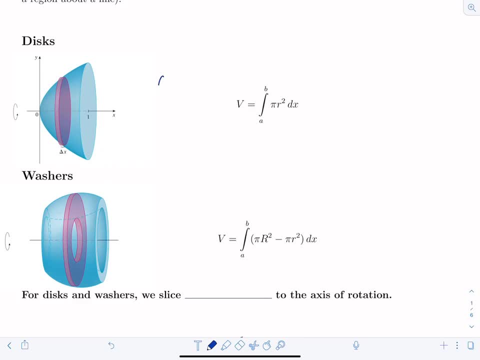 So if you look at one slice here, okay, we can see that there's no holes or gaps in it. This is some arbitrary slice. The thickness is delta x, which is dx in the integral. And then the area is going to be, well, it's a circle, right, since I'm revolving around the x-axis. And we know the area of a circle is pi r squared. So that's where we come up with the volume formula here for a disk. 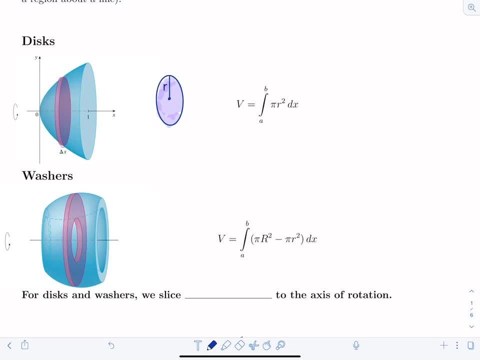 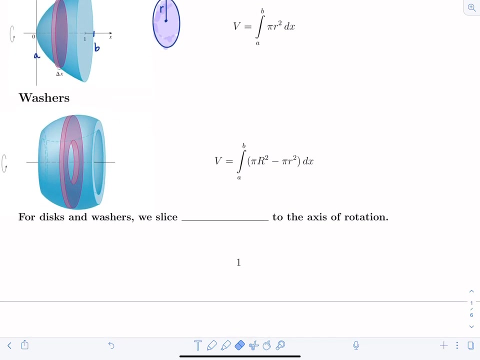 I have the integral, I have the volume, and I have the integral. So I have the integral, from a to b, assuming that the volume or the solid is bounded between a and b, whatever they may be, times pi r squared, since that's the area of some arbitrary slice dx. Now r needs to be in terms of x. So we'll look at different examples how exactly to do that. Now a washer occurs when the region that you're revolving creates a hole in the middle. So when each cross-sectional slice looks like a washer. 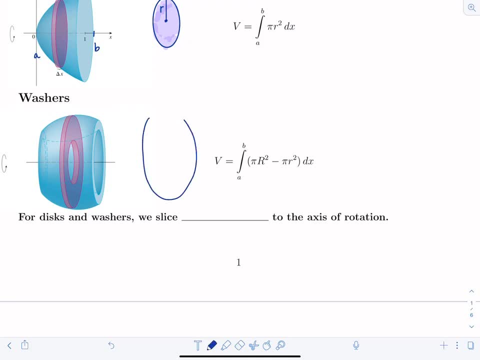 Donuts are more fun. So if you were to look at a slice here, 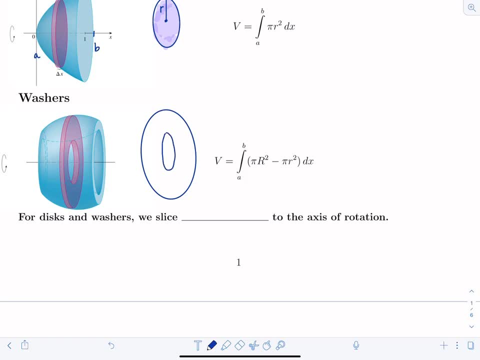 you're gonna have a circle on the outside, and then a hole in the middle. So you have two radii. This is what the area of one slice would look like. Well, how would you compute this? Well, how would you compute this? Well, you have this outer radius from here to here, this we'll call capital R, some books just say r with subscript x. capital R. Some books just say R with subscript out. And then you have an inner radius, and you would need to subtract that out, yes? Because that's the hole that's not a part of your solid. That's little r. So the purple shaded area would be the outer circle minus the inner circle, which is why you have pi times capital R squared minus pi times lowercase r squared. 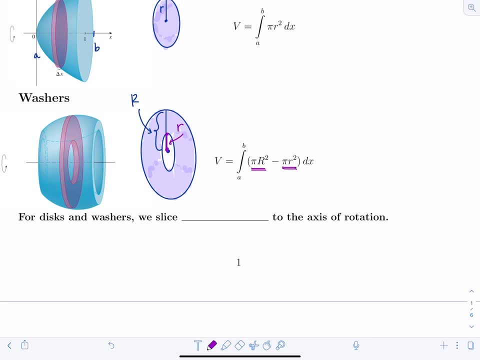 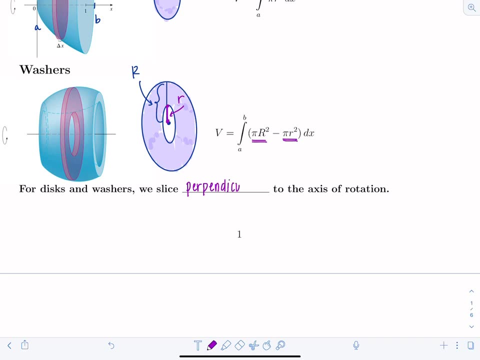 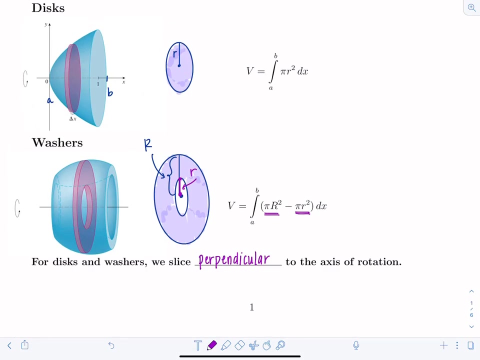 Again, integrating from A to B, dx. Now for disks and washers, we slice perpendicular to the axis of rotation. Meaning for both these examples, these integrals were set up with respect to x, right? dx. All those slices were taken in the x direction, and that's because we're spinning around the x-axis. So perpendicular to the x-axis is slices in the x-direction. If we were spinning around the y-axis, and we were using the disk or washer method, we would be spinning around the x-axis. So perpendicular to the x-axis is slices we would integrate with respect to y. And we're going to consider examples doing both directions, okay? All right, so here we go. Let's look at an example. 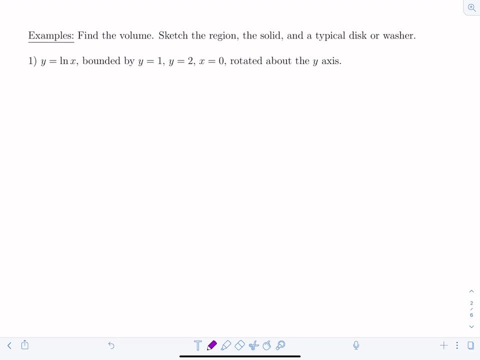 Find the volume, sketch the region, the solid, and a typical disk or washer. That's kind of like how we used to sketch a typical rectangle, same idea. So here, the first one is y equals the natural log of x. And then we're going to integrate with respect to y. And we're going to find the volume, sketch the region, the solid, and a typical disk or washer. That's kind of like how we used to sketch a typical rectangle, same idea. So here, the first one is y equals the natural log of x. And then we're going to integrate with respect to y. And we're going to find the volume, sketch the region, the solid, and a typical disk or washer. That's kind of like 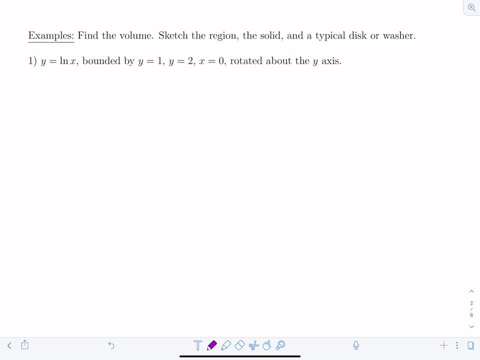 it's bounded by the horizontal lines, y equals 1, y equals 2, the vertical line x equals 0, aka the y-axis. And we're rotating this about the y-axis, okay? So before I begin, I want to know how to scale things out on the x-axis. I know in the y-axis, I'm really focusing just on the area 1 and 2. But how far do we need to go on the x-axis? Well, if it's bounded by 1 and 2, let's see. If y equals 1, that means the natural log of x would be equal to 1. So in that case, x would be e, which is about 2.7. And then if y is equal to 2, that means natural log of x equals 2. So x equals e squared, which is about 7.4. So my x-axis, I'm going to scale it out up to, let's say, 8. And then since I'm spinning around the y-axis, I'm going to scale it out up to, let's say, 8. And then since I'm spinning around the y-axis, I'm going to scale it out up to, y-axis, I'm going to go down to negative eight as well. All right, so here's the y-axis and the x-axis. I'll put it here, maybe a little bit more. 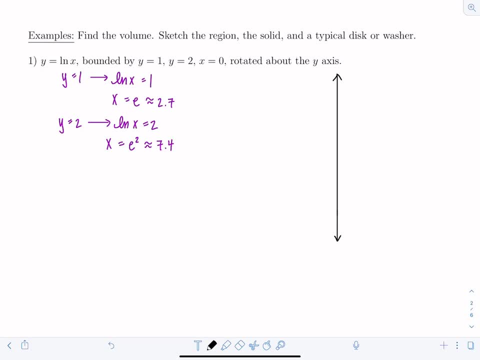 Okay, so we're going to go out to eight. Actually, I need more. 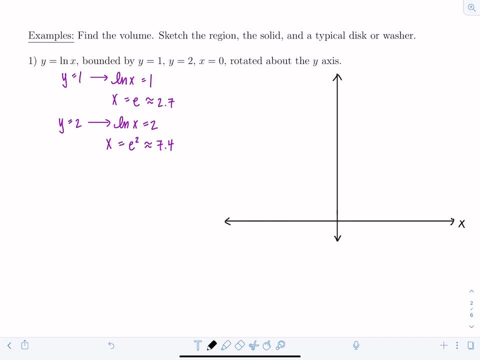 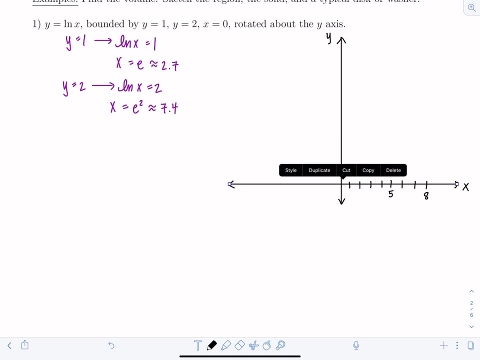 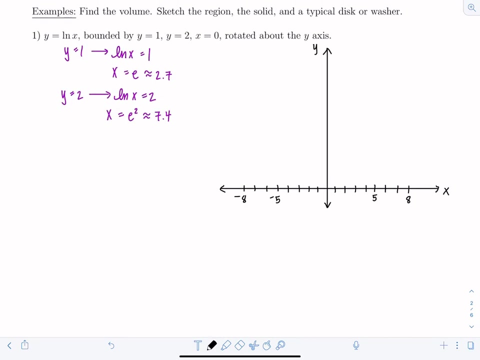 Much better. Oh, yes. Okay, here's the x-axis, y-axis. Now, let's go out to eight. One, two, three, four, five, six, seven, eight, and negative eight. One, two, three, four, five, six, seven, eight. Okay, and then y, I'm only interested in focusing between one and two mostly, so I'll spread that part out nicely. So let's say this is one, this is two, three. Okay, so we have y equals natural log of x bounded by y equals one, if y is one, x is 2.7, so right here, and then if y is two, x is about 7.4, so right around here. So I'm only interested in this portion of the graph of ln of x, and then I'm also bounding it by x equals zero. So here's y equals one, here's y equals two, and then x equals zero is the y-axis, that's bounding it. So can you see what the region is? That we're going to spin? This is the region. It has to be some bounded region, so they have to give you enough curves that it creates this closed region. 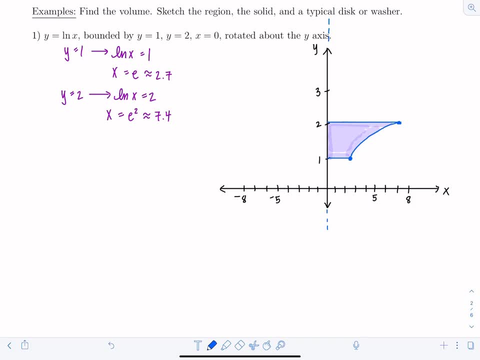 And I'm going to be spinning or revolving this around the y-axis. Okay, so now let's see, what would it look like if we spun this region around the y-axis? You basically can sort of reflect it over the y-axis. I'm going to draw the part that results from revolving it just in gray, so that you know it's not part of the original region, okay? 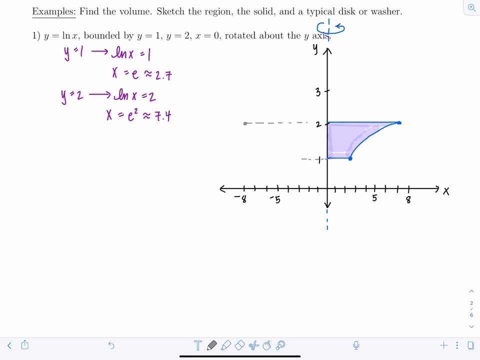 So here on the other side, if we revolved it, okay, and then this part would be rounded at the top, and then we're going to draw a typical disc or washer. Well, it's going to be a disc, it's solid. Let's make this darker, it looks so sad. Good. Okay, so a typical disc... Remember, we're going to take slices perpendicular to the axis of revolution. 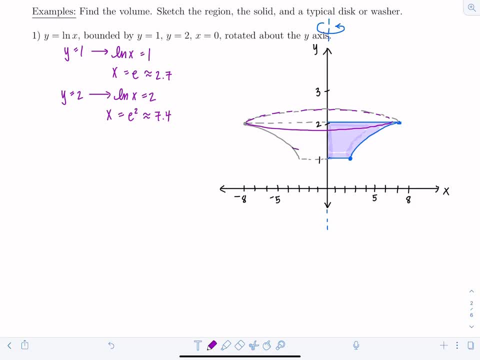 So we're spinning around the y-axis perpendicular to that. We would have a slice that looks like this. Is it solid or is there a hole in it? Is it a disc or a washer? It's a disc, right? There's no gaps in it. I'm going to color it in nice and solid. Okay, so this is a typical disc. 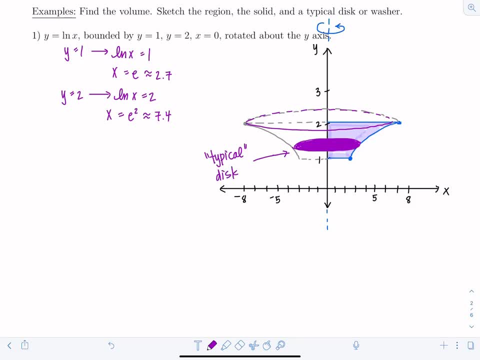 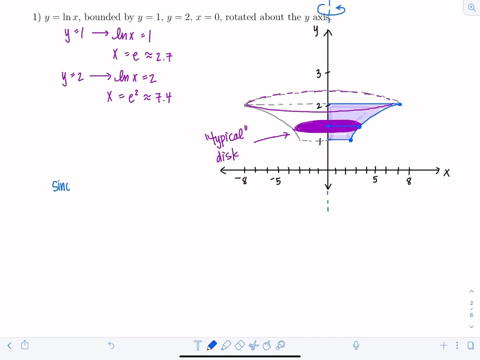 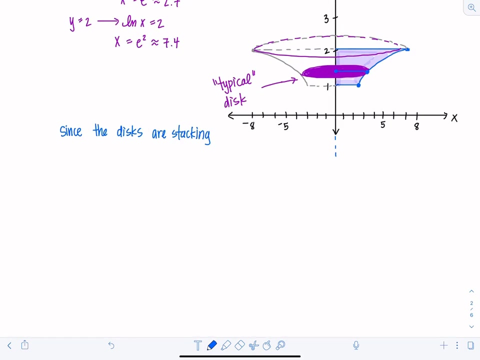 All right, well, I need to identify what the radius is. Let's see here. Well, before I do that, I want to decide if am I going to be integrating with respect to x or y. So here's the thought process. Since these discs are stacking, will you tell me which way are they stacking? Vertically or horizontally? If I'm slicing perpendicular to the y-axis, they're going to be stacking vertically. So these discs are stacking up in the vertical direction, then that means we need to integrate with respect to y. So what does that mean? We need everything in terms of y, and you get the whole set of discs. 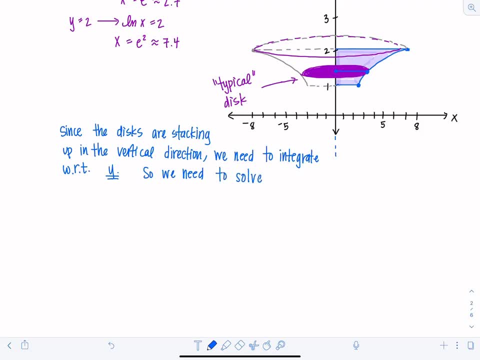 terms of y. We need to solve the function in terms of y. So y equals natural log of x. I'm going to solve it for x and x would equal e to the y. So what does that mean? 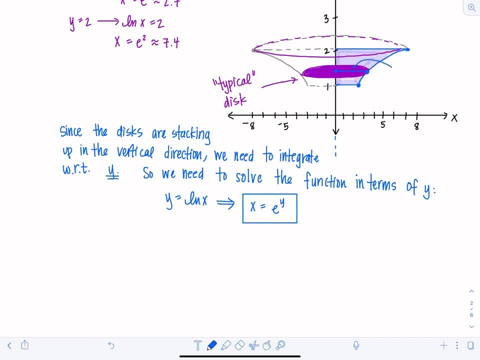 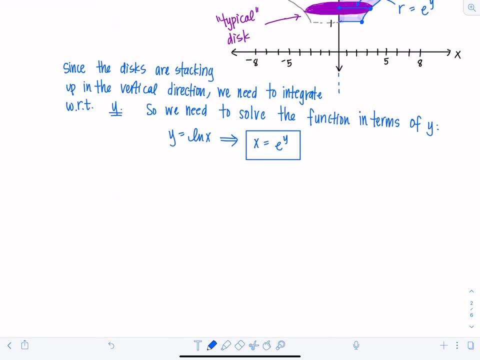 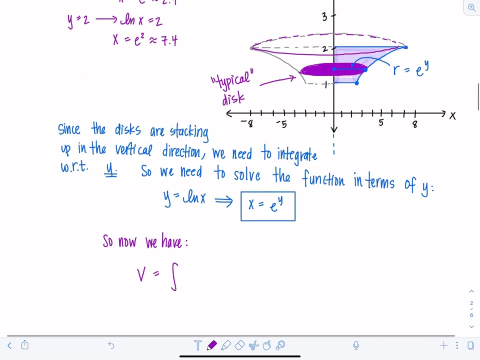 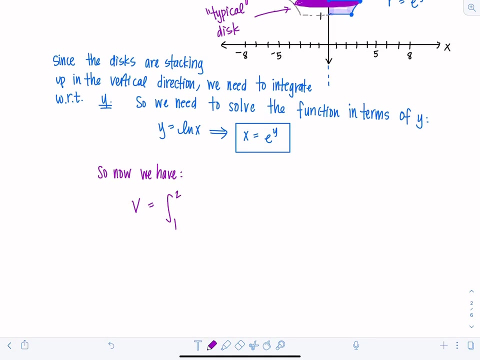 My radius here is equal to e to the y. Okay, so now I can put it all together. We have the following. The volume is going to be the definite integral. Now these limits of integration have to also match. They have to be in terms of y. So I'm going to be integrating from y equals 1 up until y equals 2. 1 to 2. And then you're going to have pi times the radius, which is e to the y squared dy. So 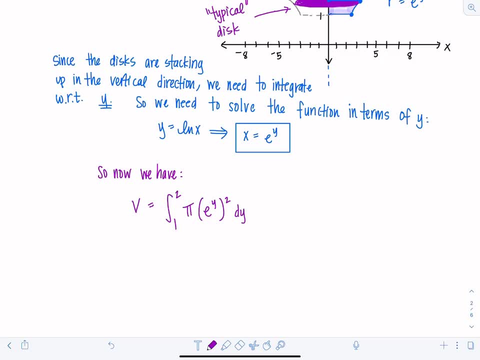 everything's matchy-matchy. Limits are y, functions in terms of y, and you need a dy. 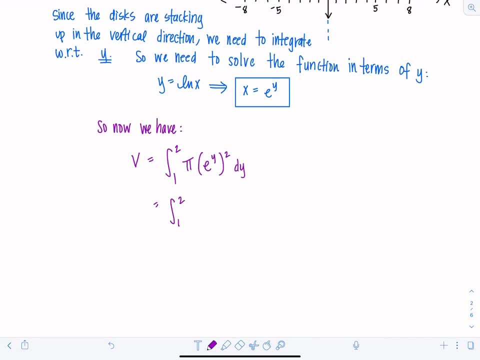 Okay, now let's anti-differentiate. So we have integral 1 to 2 pi times e to the 2y dy. 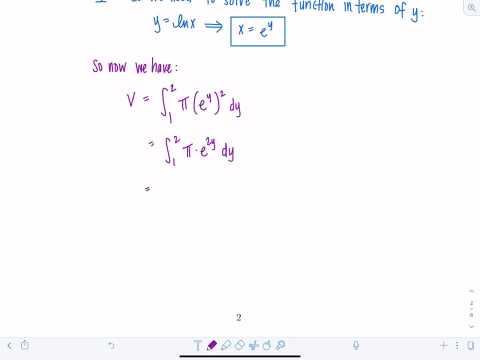 And then if I anti-differentiate e to the 2y, you can do a u-sub or hopefully you've noticed by now you can just divide by 2, right? 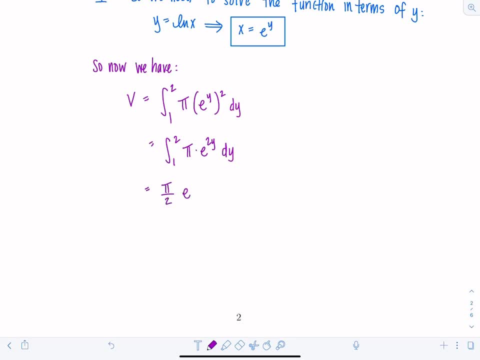 So I'm going to have pi divided by 2 times e to the 2y, evaluated from 1 to 2. And then that's going to give me pi over 2 times e to the 4th power, 2 times 2, minus e squared. 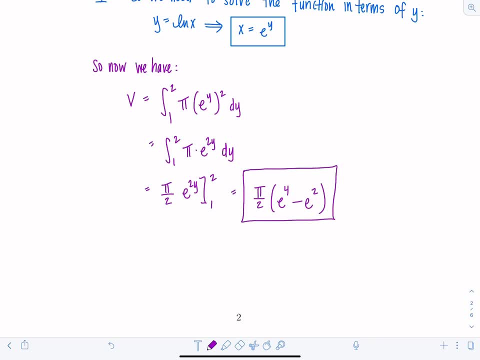 And this is our exact answer. This is the volume of that solid. So technically this is a three-dimensional quantity. You would have your units cubed on this. 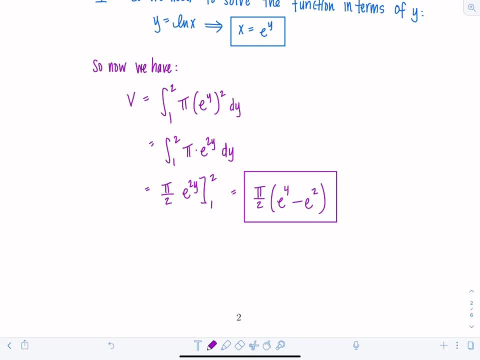 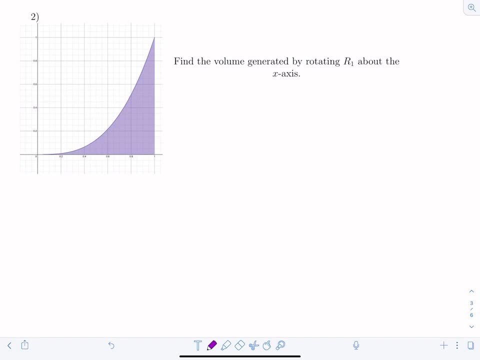 All right, nice start. Now let's move on to another example. Find the volume generated by rotating R1, this is R1, about the y-axis. And this curve is y equals x cubed, okay? So we're rotating it around the x-axis this way. 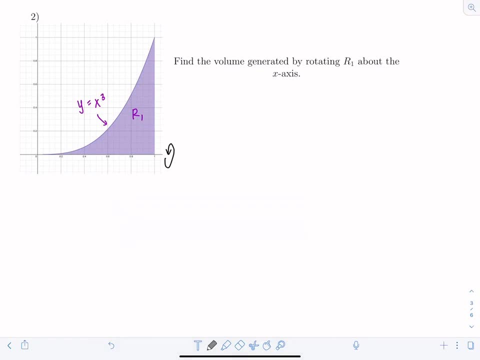 So what would it look like? Well, you can sort of just reflect it. 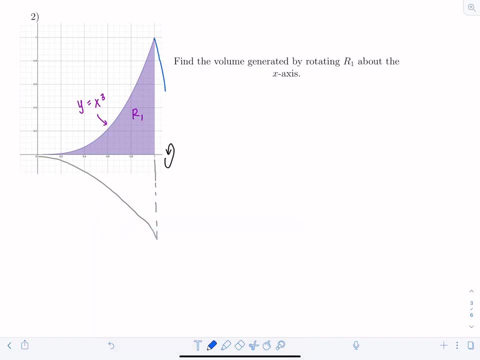 And then maybe add on a little bit, right? This would be curved over here, here and here. Here's the end of it. And if I take a slice perpendicular to the axis of rotation, I'm going to be slicing in the x-direction, right? So here's 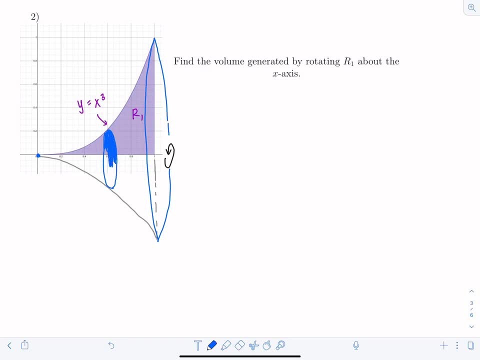 one typical slice. Is it a disc or a washer? It's a disc, right? 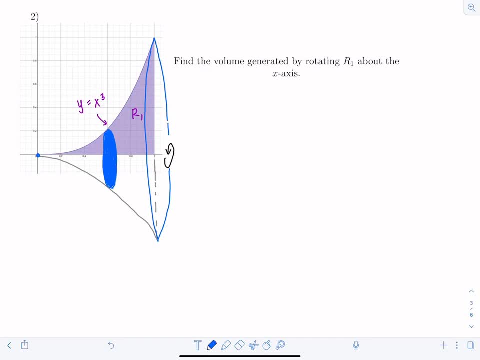 You know what this thing looks like? Have you ever played that board game, Sorry? It looks like one of those game pieces, right? On its side. 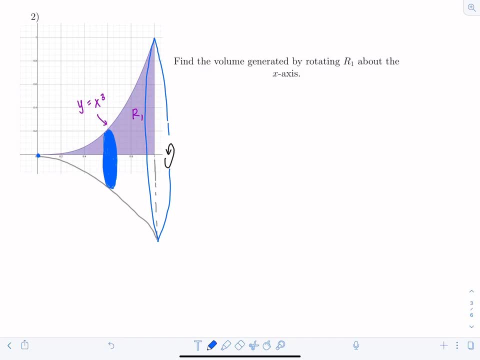 Okay, so if we're going to be taking slices in the x-direction, I need to integrate everything with respect to x. So I need to express the radius in terms of x also. Well, that's fine, because they already gave me the function. It was x cubed. So here's the radius, r equals x cubed. 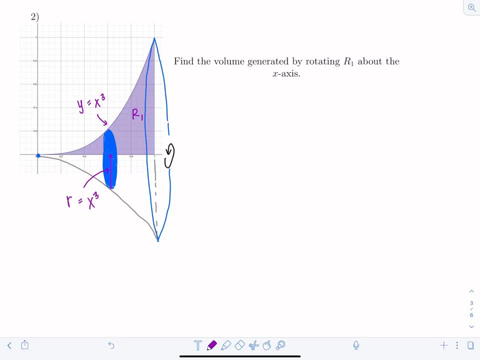 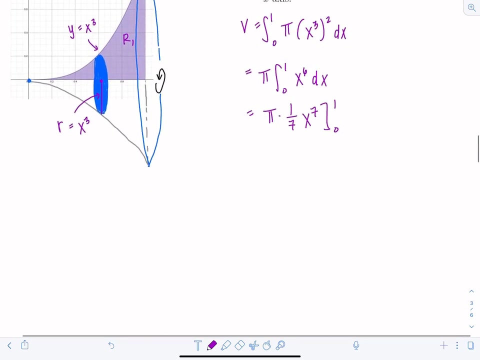 Okay, so here we go. The volume is going to be the integral. What are the limits of integration? From 0 to 1 of pi r squared. So x cubed squared dx, okay? A lot of the times I like to just take the pi outside the integral so I can focus on all the other action. So I'm going to have x to the 6th dx. So that's going to be pi times 1 7th x to the 7th evaluated from 0 to 1, which is just going to be 1 minus 0. So I have pi over 7 for our answer. 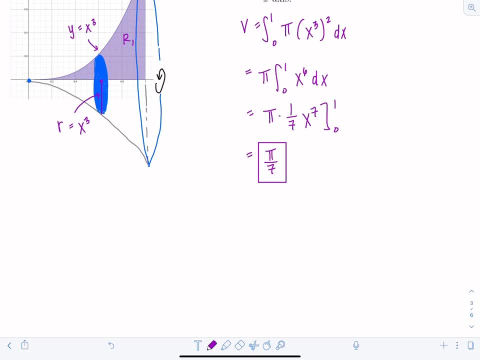 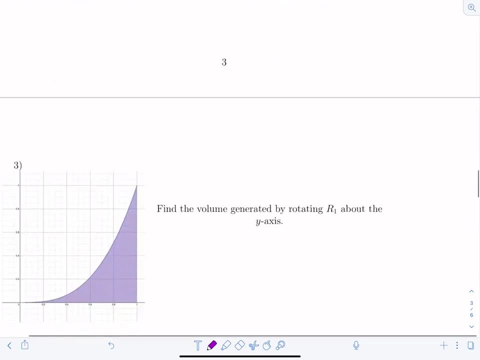 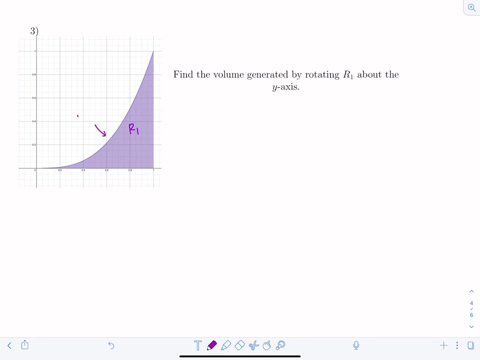 Okay, not too bad, right? Now, what if I take the same region and I change the axis that I'm revolving it around? So example 3, now find the volume generated by rotating, this is still r1, with y equals x cubed about the y-axis. 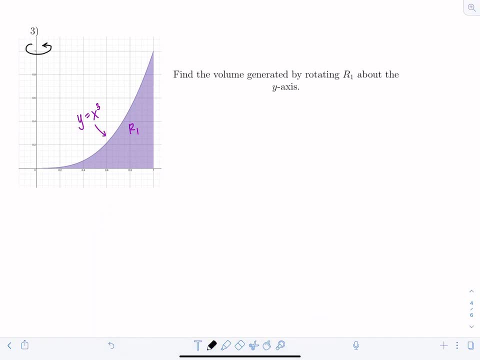 So now we are spinning this way. Okay, well, in order to draw what the solid would look like or to sketch it out, I'm going to make a separate graph over here because I need to go into the negative y direction, right? So here we have x-axis, y-axis, negative y-axis, negative y-axis, y-axis. This is 1, this is negative 1, this is also 1. Okay, so here's the region, the original region. 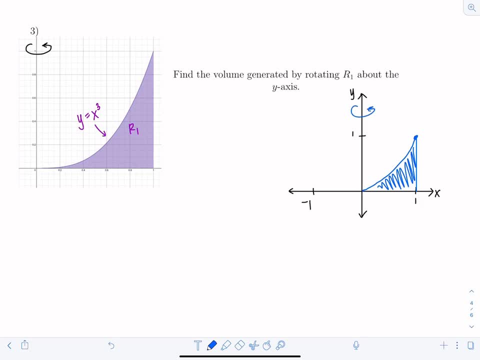 And then we spin it around the y-axis. So what does it end up looking like? 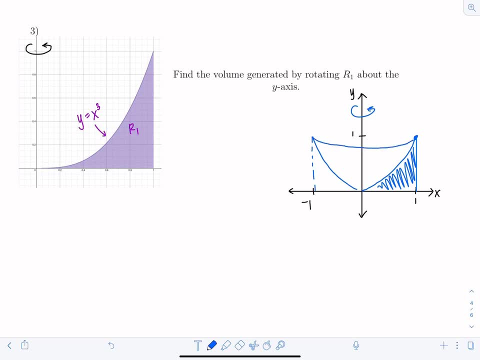 Kind of like a bowl, right? But a weird bowl. 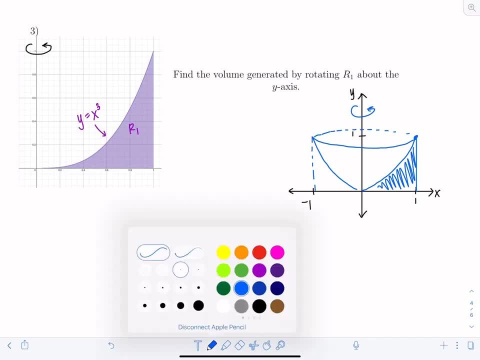 It's hollow inside. This is the part that comes from revolving it. Okay, and then now we're going to take a slice perpendicular to the axis of revolution. So I'm going to take a slice this way. 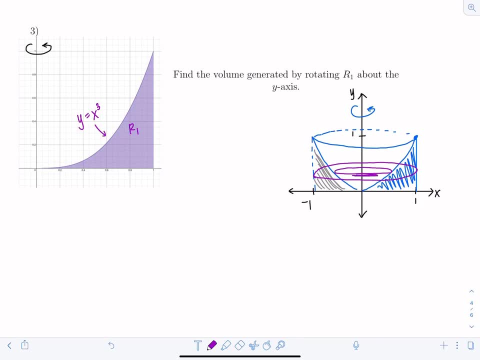 And notice now, this is the first example we've looked at where we have a washer, right? 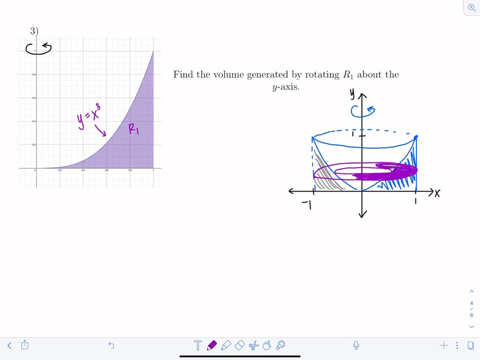 So we have an inner radius and an outer radius. So we have an inner radius and an outer radius. So we have an inner radius and an outer radius. Okay. I'm going to color it in very thoroughly. It's therapeutic and it looks good. 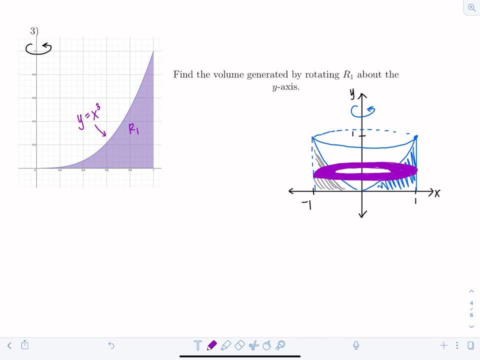 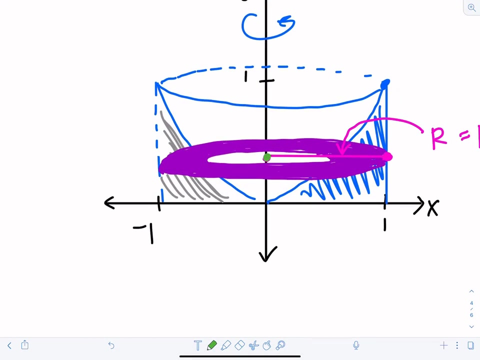 All right, here we go. Now, what is that outer radius? Let's see. The outer radius is going to start from the center and go all the way to the edge of the graph. Is the outer radius changing? Now, look at it. If I took a slice somewhere else, would it be different? No. The outer radius is always equal to one in this case. Now, what about the inner radius? The inner radius, let's zoom. The inner radius would start at the same place and then it would only go up to here. Or if I took a slice somewhere else, maybe it would go from here to here, right? So the inner radius is changing and it's changing based on whatever the curve is. So the inner radius is changing based on whatever the curve is. So the inner radius is changing. However, which way are we going to be integrating with respect to what variable? 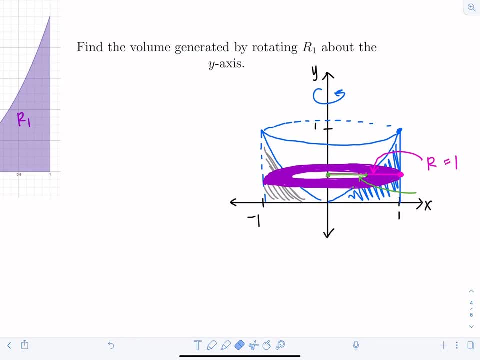 Well, remember, if I'm revolving around the y-axis, I have to take slices perpendicular and those slices are going to stack vertically. So that means we need to integrate with respect to y. 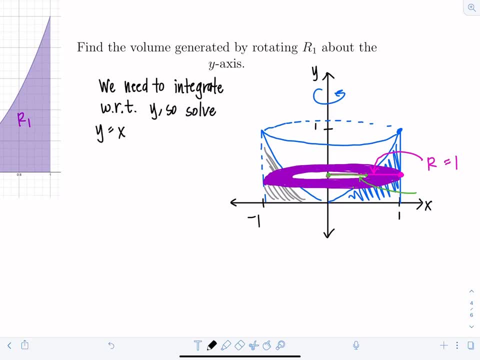 So I need to first solve y equals x cubed for x, which would give me x equals y to the one third. And then now I could say, aha! My inner radius is y to the one third. 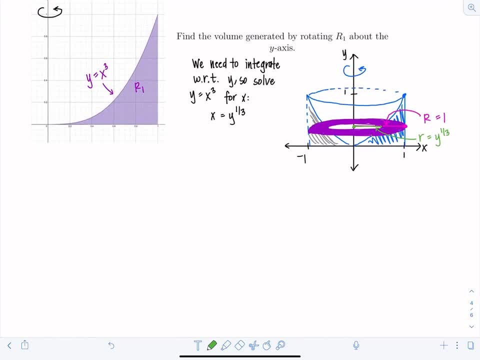 All right. So now we can put everything together in our integral. 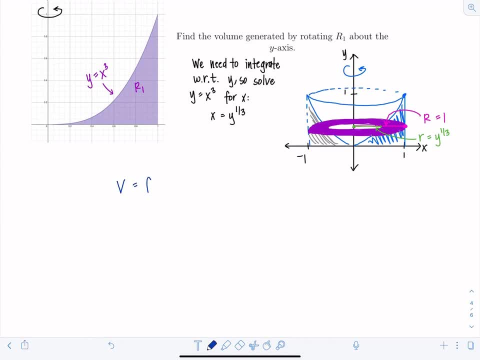 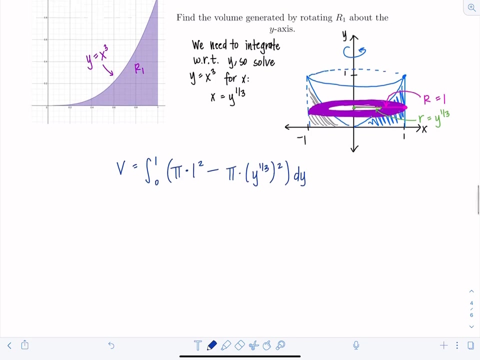 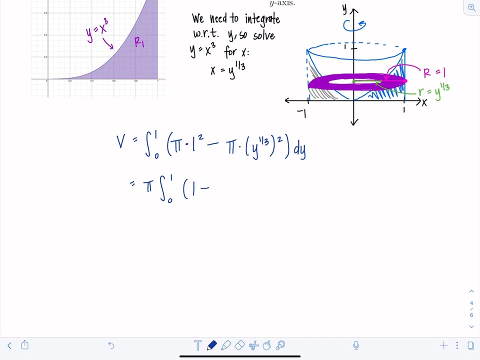 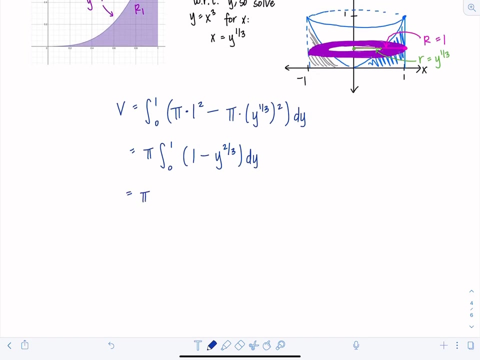 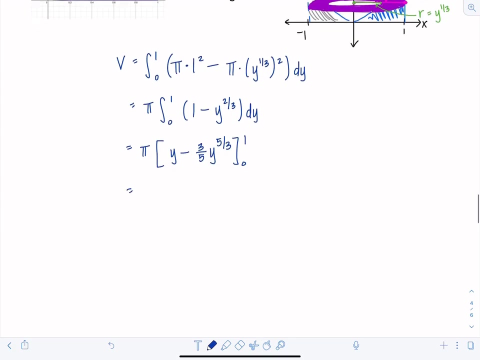 So I have the volume equals the integral. Now the limits are going to be with respect to y based on the original region that we are revolving around. so the limits are going to go from 0 to 1 and then remember we have pi times the outer radius squared minus pi times the inner radius squared dy now you don't need to put the pi next to each of those ever again just pull the pi outside it makes life easier and then you have integral from 0 to 1 this is going to be 1 minus y to the two-thirds dy and then anti-differentiating from here we have 0 times and not 0 just pi times anti-derivative of 1 is y minus this is going to be three-fifths y to the five-thirds evaluated from 0 to 1 so then this is pi times 1 minus three-fifths minus 0 so I have 1 minus three-fifths that's two-fifths times pi so two-fifths pi all right very nice 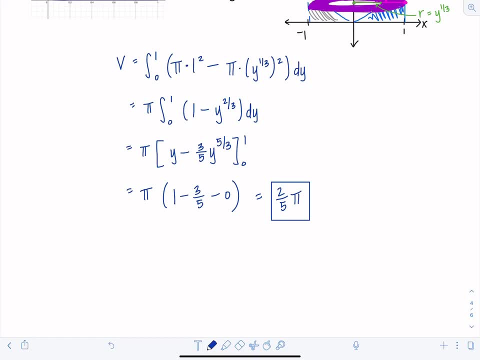 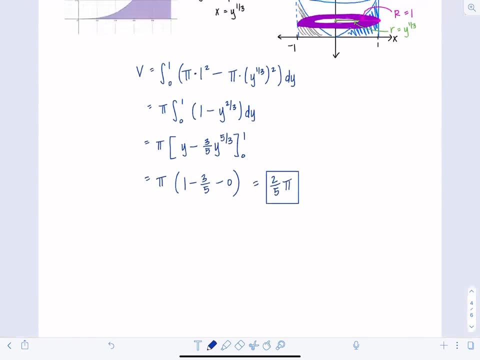 let's take it to the next level now let's spin around something other than the x or y axis once you wondering are these the only axes we're going to spin around so here we go example four we're taking the region bounded by y equals x cubed y equals one and x equals two and I'm spinning it around y equals negative three okay so let's see here what is this graph gonna look like so y equals x cubed I know what that looks like I'm only interested in the 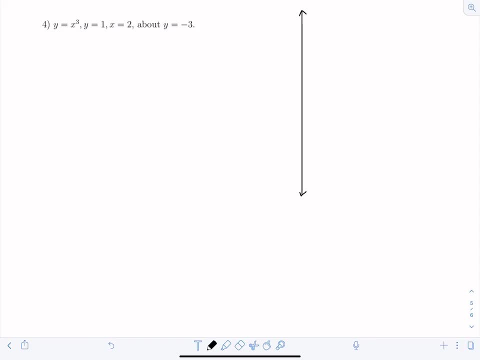 portion bounded by y equals one and x equals two and x cubed okay so here's the x-axis here's the y-axis so I won't go too far in the x-direction 1 2 sound good but if X is 2 X cubed is going to be 8 so I gotta go at least that high 1 2 3 4 5 6 7 8 and then 1 2 3 4 5 6 7 8 down there somewhere okay so let's see y equals x cubed and I'm also bounding it with y equals 1 so that would be at 1 1 and then when x is 2 y is 8 so we're bounding it here with x equals 2. and then here's y equals x cubed and then I'm also bounding it with y equals 1. okay so this is the region that's going to get spun okay 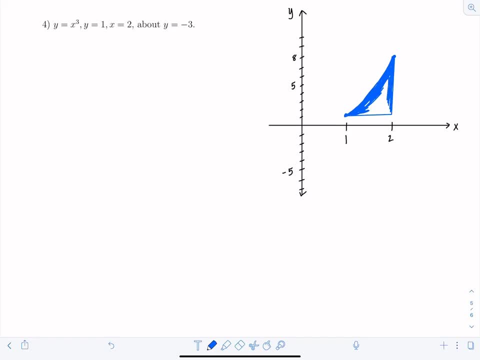 now notice in this case we're spinning it around the line y equals negative 3 so I'm going to color this in and then show you what that's gonna look like so y equals negative 3 where's that one two three right here y equals negative 3 we're spinning around this okay so there's gonna be a gap in the line y equals negative 3 and then there's gonna be a gap in the line x equals negative 3 over here. 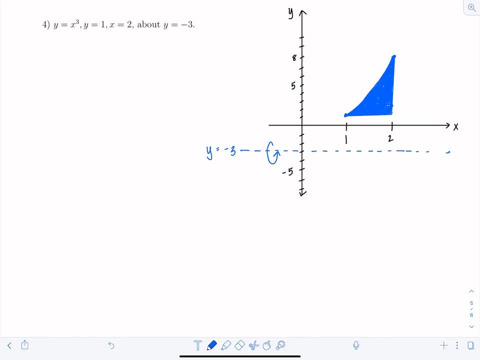 middle right how big is the gap well look this is one unit above from that so this is four units so i'm gonna go down another four units before i reflect what i have so one two three four i'll do it in gray because this is not part of the original region right this is just a result from 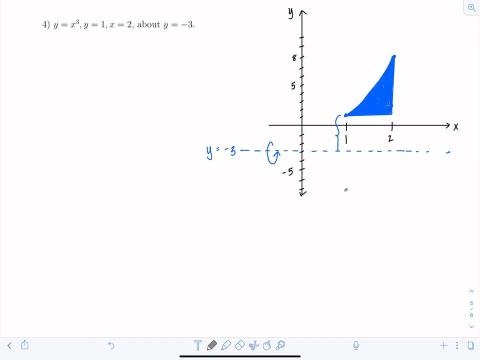 revolving so one two three four here just mirror it just mirror it about that axis okay it's gonna be something like this like this right and then we have to decide which way are we going to be 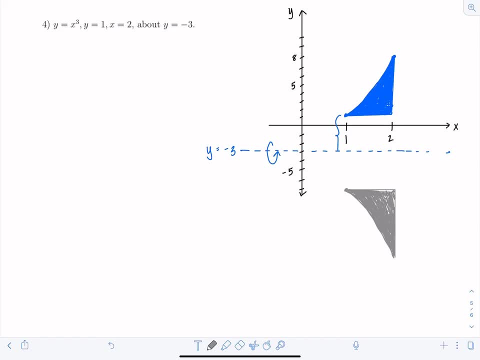 slicing to so if we're spinning around y equals negative three slices perpendicular to that axis are going to be stacking in the x direction right so you're going to have a piece here like this 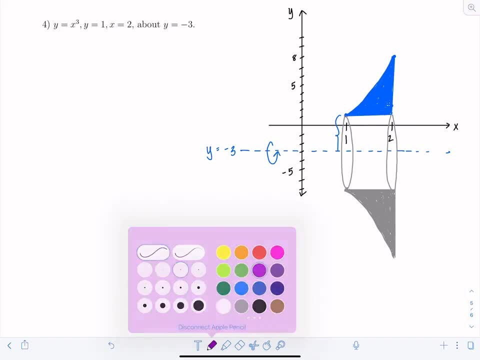 and over here and let me take an arbitrary slice so we've definitely got a washer right 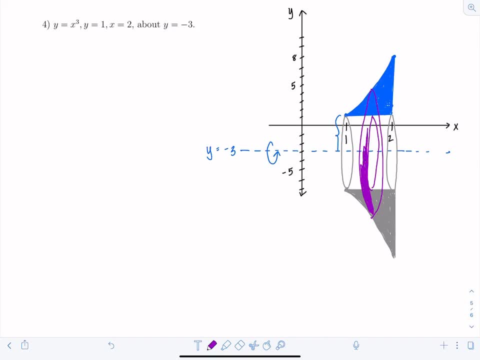 okay now we have to determine what the inner radius and what the outer radius are okay so let's first focus on the outer radius 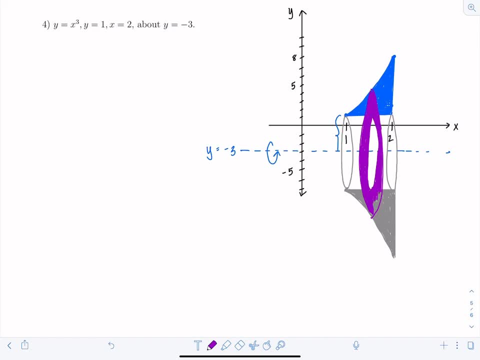 so okay so let's pick up the orange here because this part is the larger part it's therapeutic to color so really take your time with this part 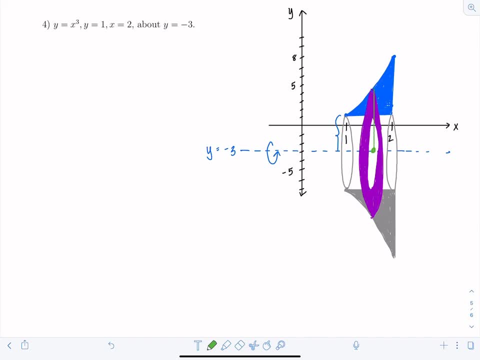 okay so outer radius let's see here that's going to be from the center to the end of the solid 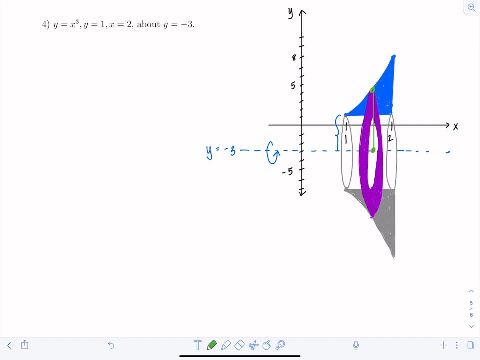 so how much is that well you cannot say x cubed because x cubed is only the distance from the x extra three units tacked on there, okay? Now you can kind of think back to when we found area between curves and you did top curve minus bottom curve. So you could think of the same thing to find the outer radius. The outer radius is going to be that top function bounding the outer radius's slice, which would be x cubed, minus negative three, since y equals negative three is bounding the inner radius from below. Or you can just look at it and say, oh, that's x cubed plus an additional three units, okay? Now what about the inner radius? Now this one's interesting because the inner radius actually doesn't change, right? No matter where you take your slice, that's the inner radius, and it's always equal to, can you tell? A cylinder of radius four is basically being drilled out of this solid. 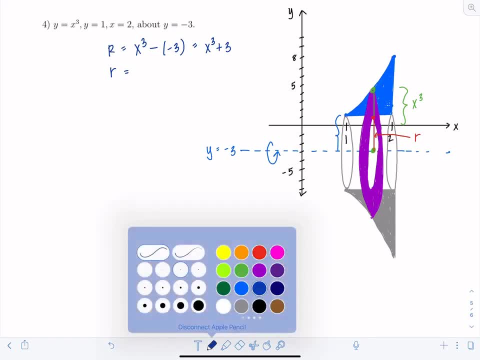 So if you want to think of it in terms of how we computed the outer radius, you would take what's bounding the inner radius above, well, y equals one, minus, we're spinning around negative three, that's bounding it below, which is four. Or you can just look and say, oh yeah, that gap is size four, that inner radius is a solid 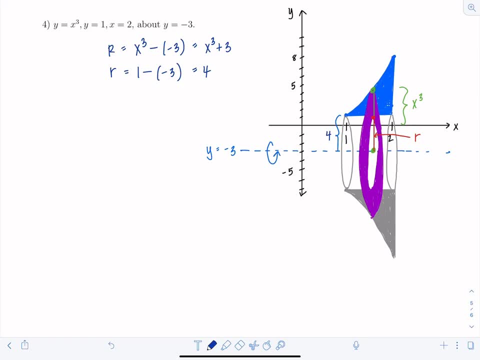 cylinder, it's not changing. No matter what the slice is, the inner radius is always four. And if you don't believe it, just draw another washer and make sure you get the same thing, right? 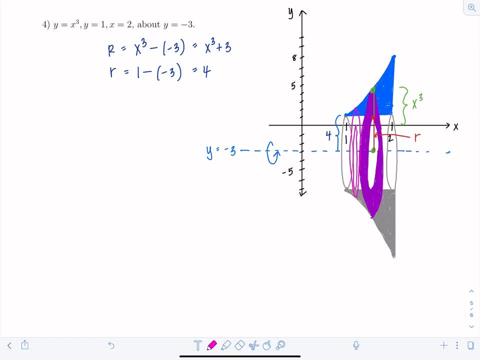 So you can see the inner radius is going to be the same. Okay, I'm going to erase it because that's looking messy. Okay, cool. And since we're spinning around y equals negative three, then we know we're integrating with respect to x. 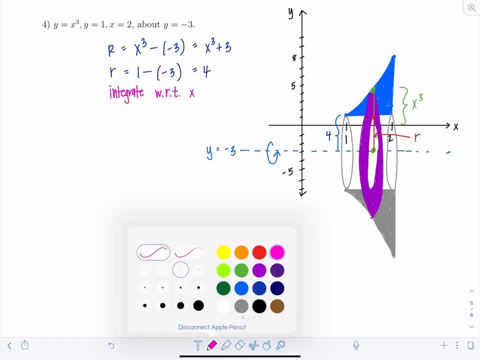 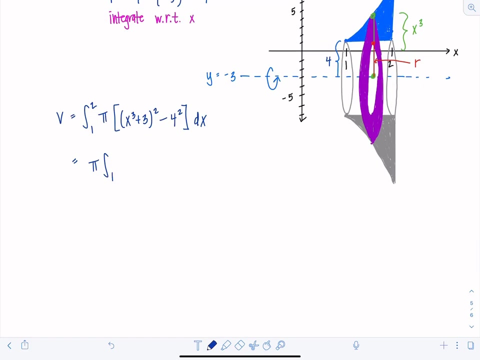 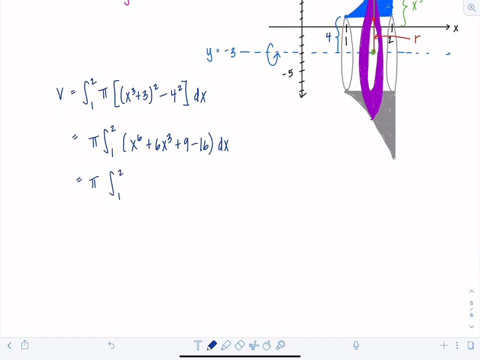 Okay, so let's set up our volume in the x direction. So the limits have to be in terms of x. So it's going to be from one to two. You can pull the pie outside, and you're going to have outer radius, squared, minus inner radius squared, dx. Okay, so this is going to give me, let's pull the pie outside, get them out of the way, integral one to two, this is going to be x to the sixth, plus six x cubed, plus nine, minus 16, dx. So this is pi times the integral from one to two, 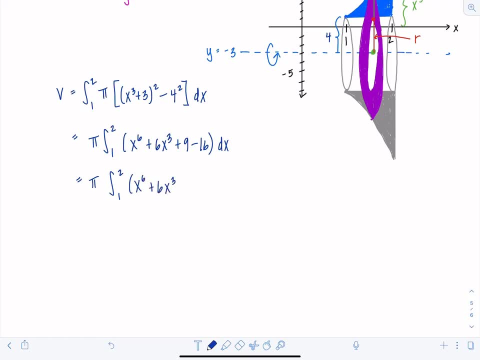 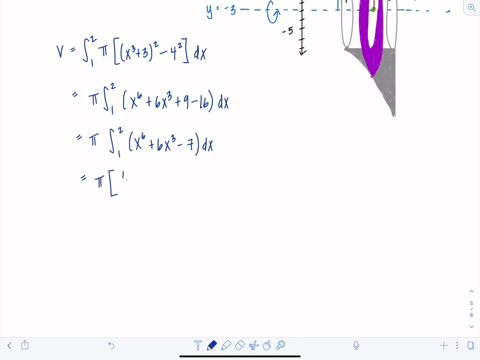 x to the sixth, plus six x cubed, minus, seven, dx, which is going to be pi times one seventh, x to the seventh, plus six over four, so three over two, x to the fourth, minus seven x from one to two. And then now I'm going to evaluate the limits of integration. So I have pi outside, two to the seventh, that's 128 over seven, 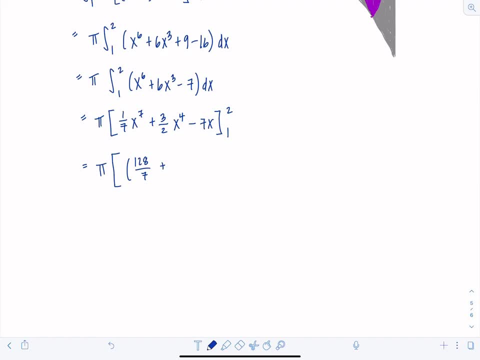 plus two to the fourth, that's 16 times, three is 48, divided by two, 24, minus 14, minus, if I plug in one, now I get one seventh, plus three halves, minus seven. Okay, and then this is 471 pi over 14 units cubed. Oh, how cute, I'll take it. Okay, 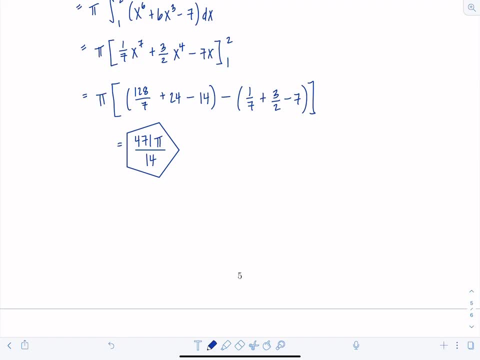 how are we doing? One last one, hang in there. You'll be excited when you see the directions. 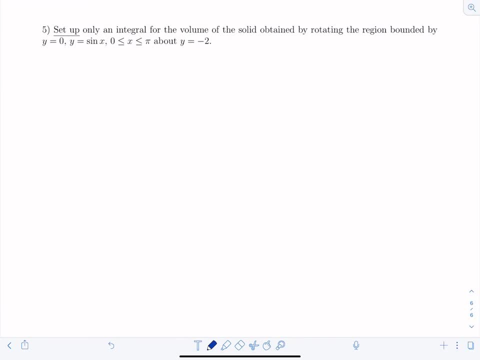 Look, set up only, so you don't have to evaluate it, an integral for the volume of the solid obtained by rotating the region bounded by y equals zero, aka the x-axis, y equals sine x, 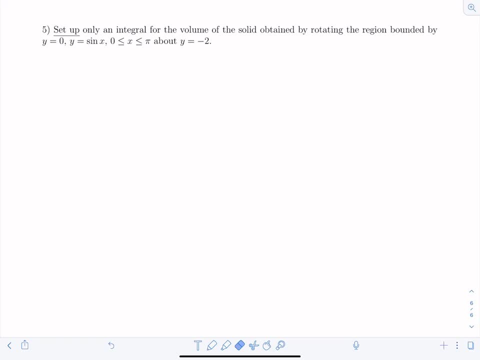 they're already telling us x is between zero and pi, and we're spinning it around y equals negative two. So kind of similar to the last one, we're spinning around a horizontal line. 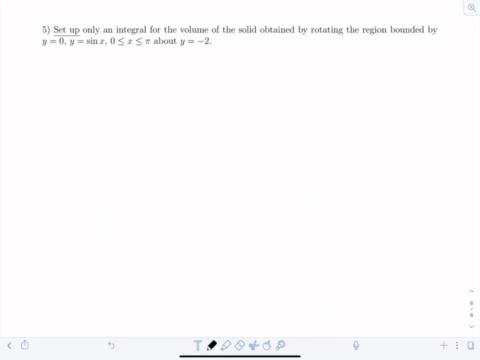 Okay, so if I'm spinning around y equals negative two, I know there's going to be like a hole in the middle of this, or a cylinder drilled out most likely. 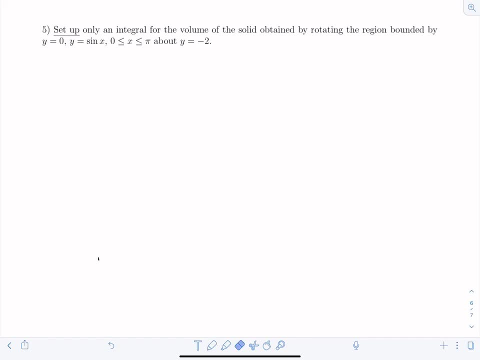 So I'm going to put a lot of my graph in the negative y direction. Oh, you know what, it doesn't want to draw over there. 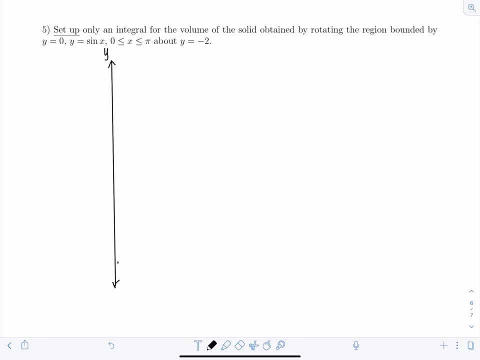 Good. Okay, so here's the y-axis, and then I'm only going to go up to, a little past one, right, because it's sine x, it's not going to go up very high. 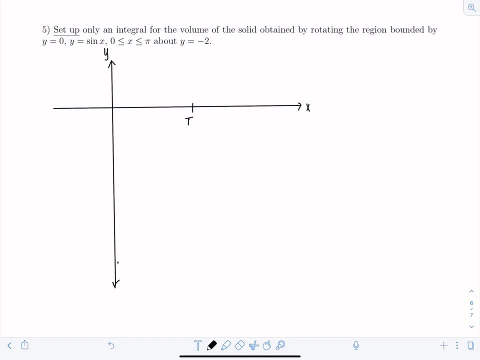 Here's the x-axis. We're only interested in the area from zero to pi. So here's one, and then we're spinning around y equals negative two, spinning around this. Okay, so perpendicular to y equals negative two, the slices are going to be stacked in the x-axis. Ohh! 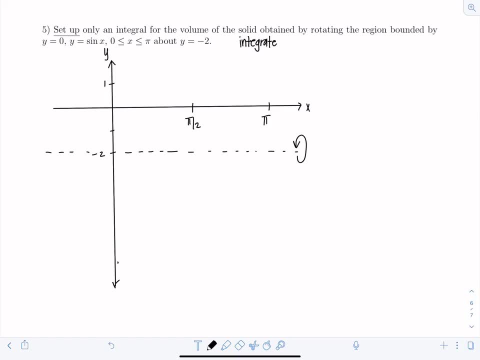 Alright, so I think that's the x direction, so I'm going to integrate with respect to x. 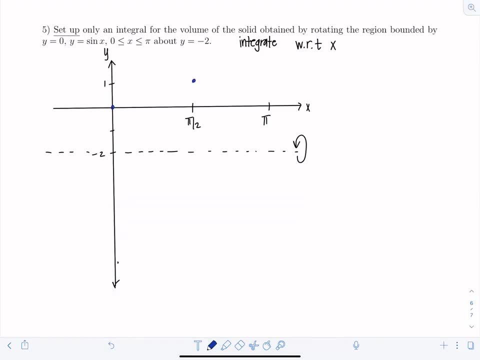 Okay, so now let's graph sine x, so zero, zero, pi over two, one pi, zero. We also bound below by the x-axis. 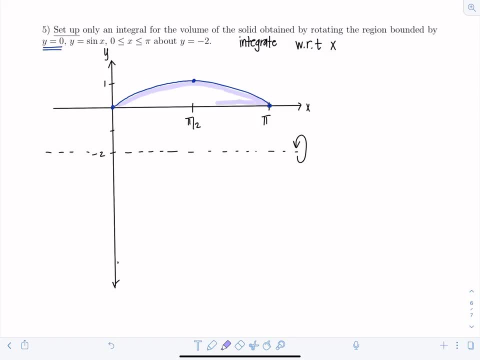 So what are we spinning? We're just spinning this region here. 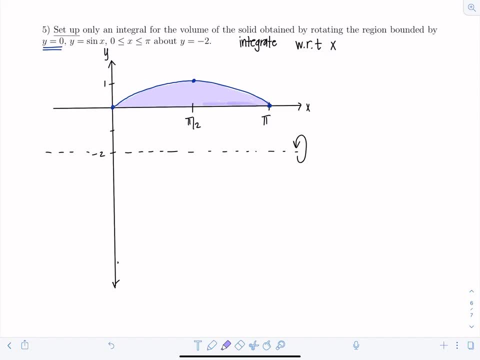 Okay, and I'm spinning it around, y equals negative two. So look, I have this gap of two units, so I'm gonna mirror it on the other side. Okay, so this is the result from revolving. 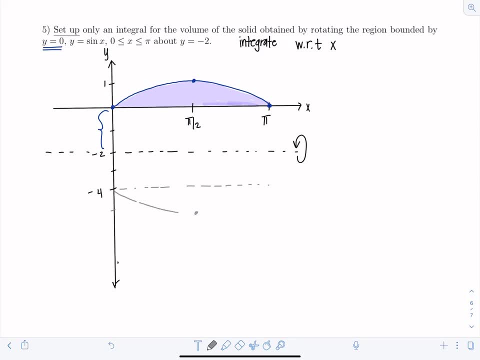 And then I'll go down to negative five there. 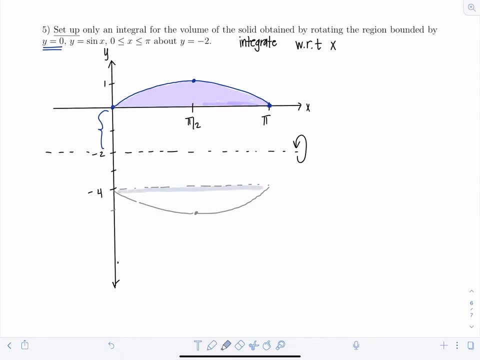 And let's change this up so it's gray as well. Since this was not part of the original region, right? So this is just the result from revolving. 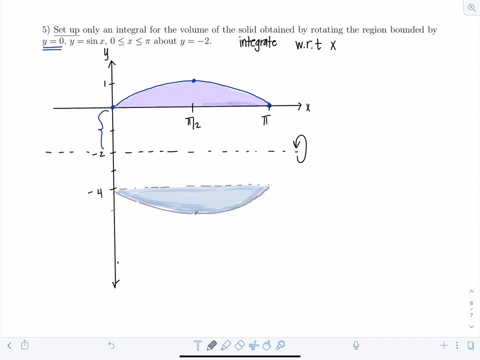 Okay, so what would our solid look like? Well, you could kind of close up the ends of it, right? So there's that cylinder missing in the middle. 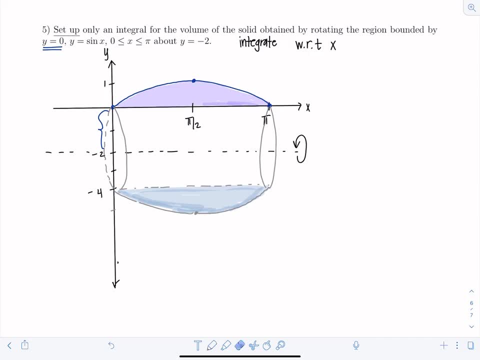 Okay, so let's take a slice perpendicular to the axis of revolution. So I'm gonna draw a slice here. And we can see we have a washer, 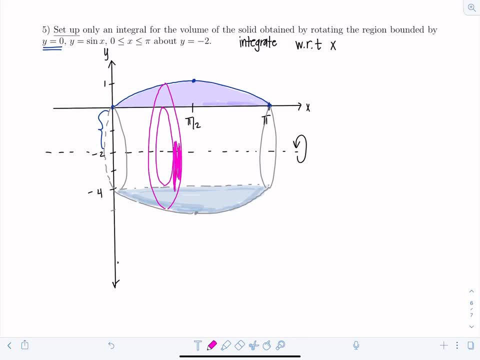 so I'm gonna have an outer radius and an inner radius. And now let's see if we could figure out how to express that outer radius in terms of x. 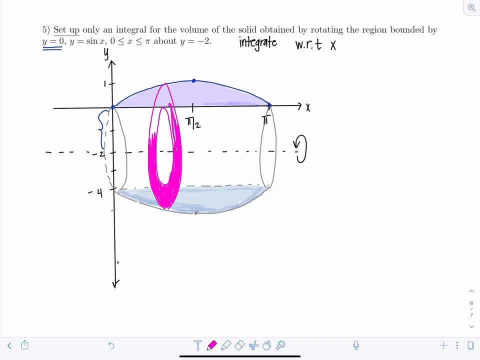 Okay, the coloring time is the time to regroup, you know? 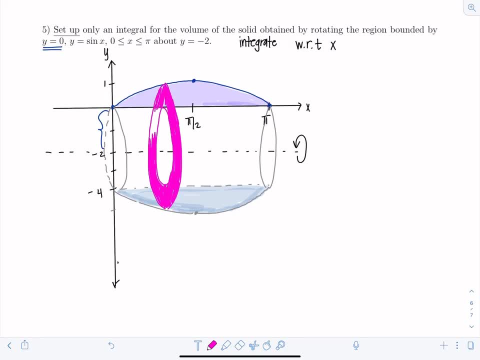 Go, all right, I'm gonna plan my strategy, have a nice picture that way. Do a good job. 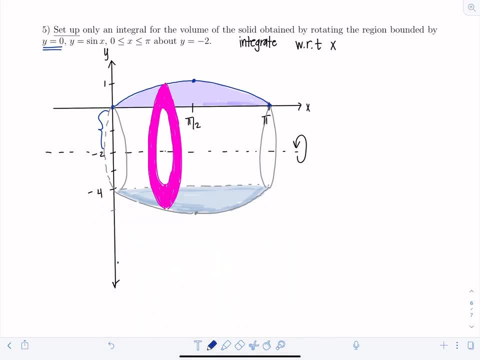 All right, outer radius, let's see here. So it's gonna start from the center, go all the way to the outside of the solid. That's the outer radius. 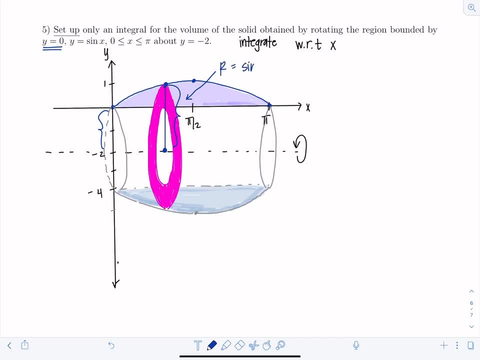 So it's equal to top function sine of x minus what bounds it below, negative two. So outer radius is sine of x plus two. 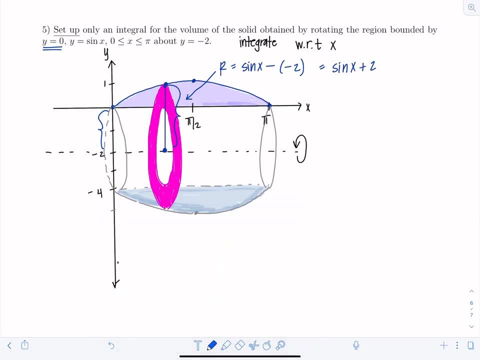 What about the inner radius? What am I subtracting out? This is the inner radius, right? Is it changing? Take another slice somewhere if you want. 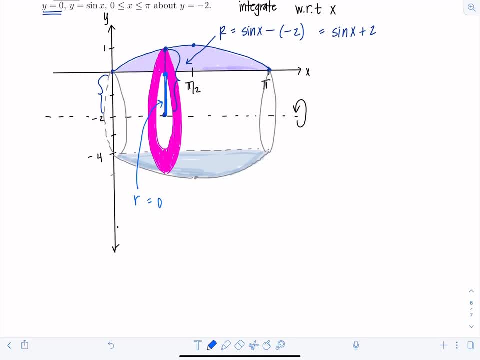 The inner radius is just equal to two. Or you could say it's the top function, which is y equals zero minus negative two. 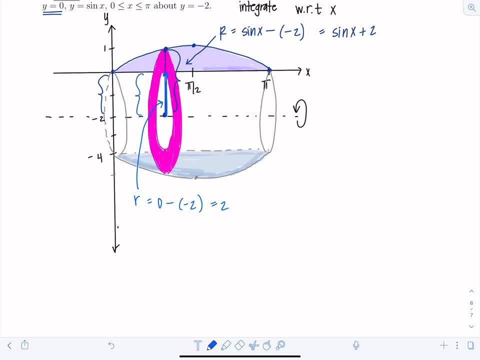 So r equals two. Or you could just look, right? Oh, I have a cylinder of radius two being drilled out from it. Okay, awesome. Now we just have to set this one up. 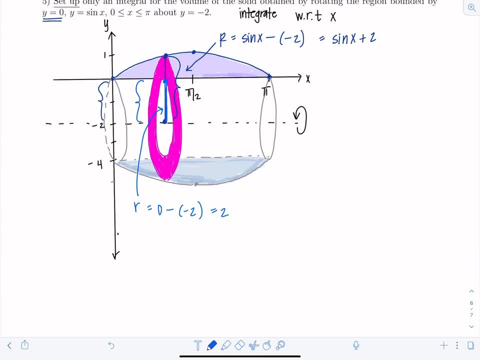 So our limits of integration are gonna be in terms of x. They're right here given to me, zero to pi. So volume's gonna be the integral from zero to pi. 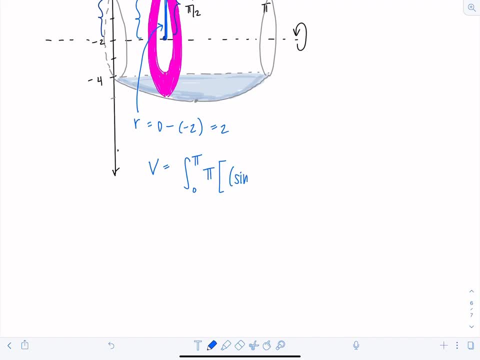 I have pi times outer radius sine of x plus two squared minus inner radius, which is two squared dx. 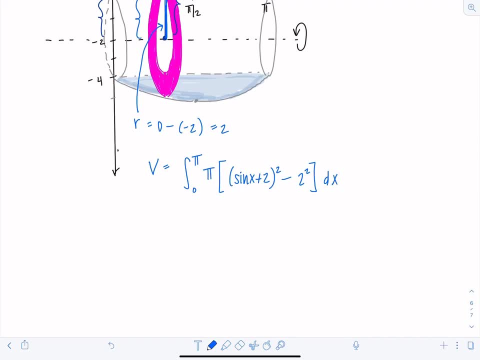 Now the problem did say set up only. So technically we've set it up. So depending on your instructor, they may or may not say you're done. 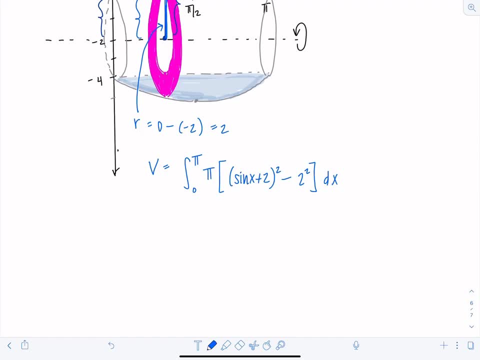 But the reason why they said set up only is because later on, you're gonna learn how to actually compute this integral.